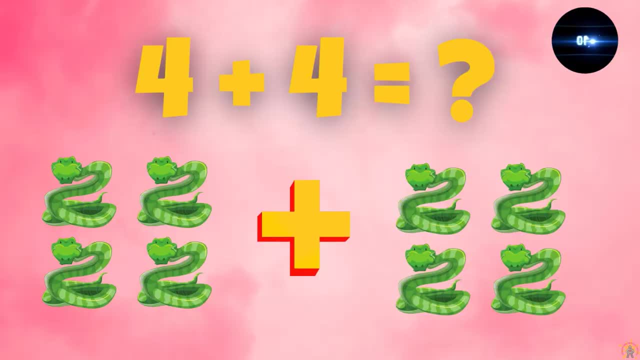 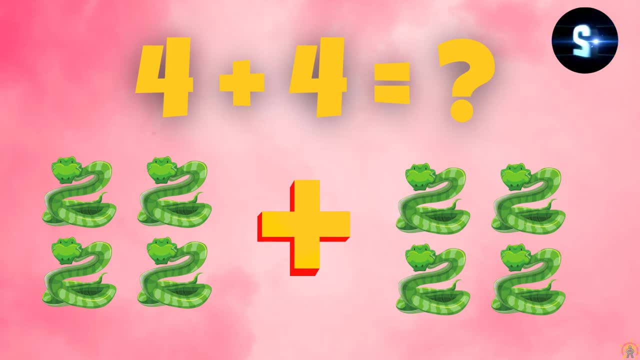 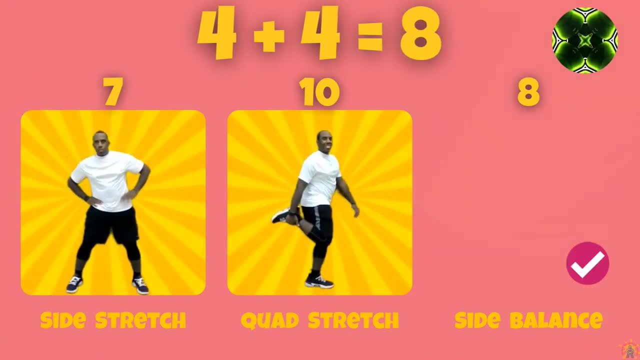 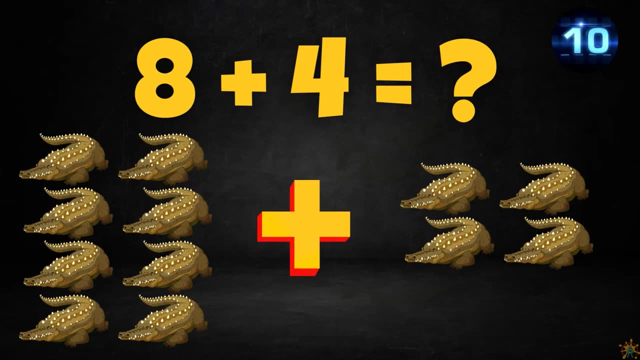 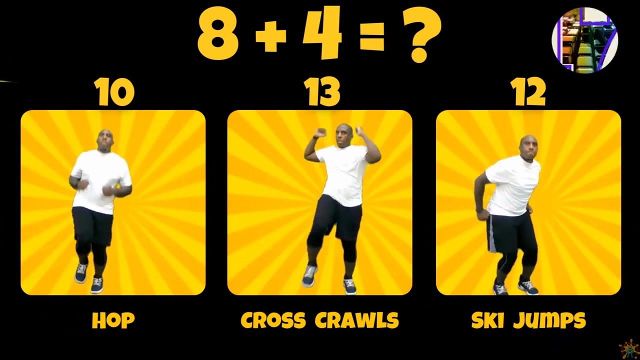 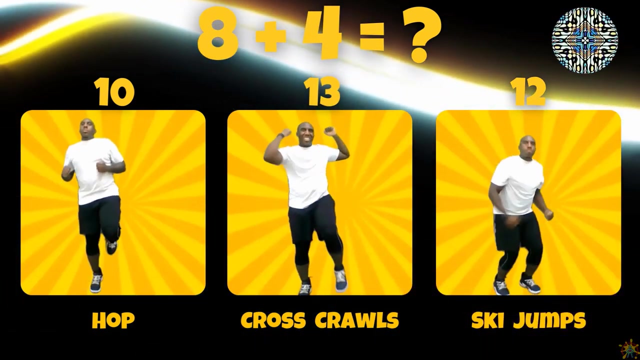 What does 7 plus 6 equal? 1. What does 7 plus 6 equal? 1. What does 7 plus 6 equal? 1. What does eight plus four equal? Does eight plus four equal ten, thirteen or twelve? 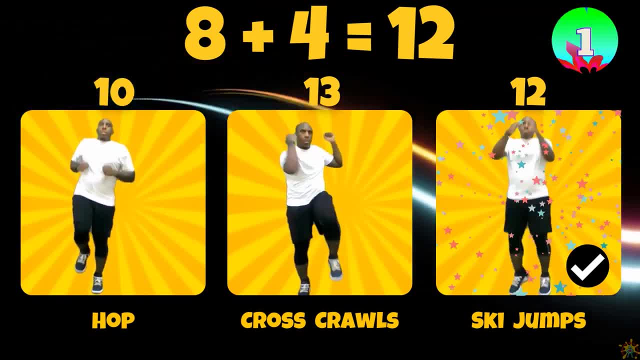 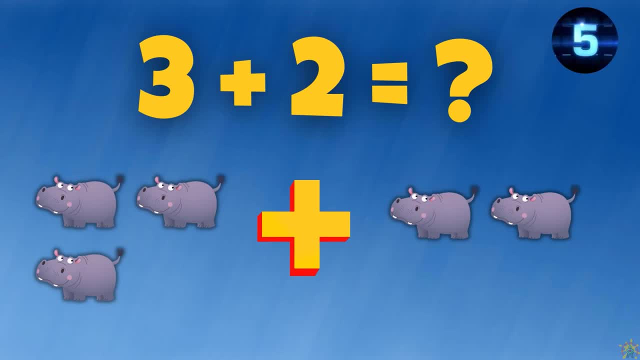 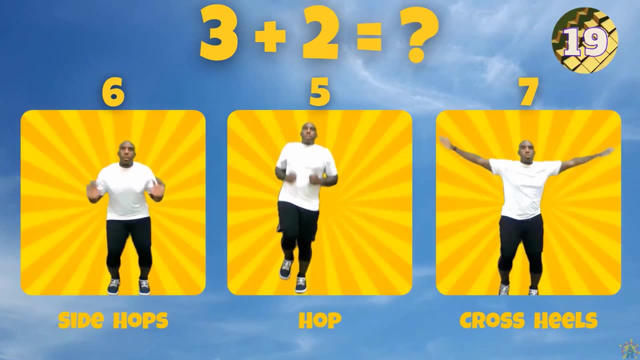 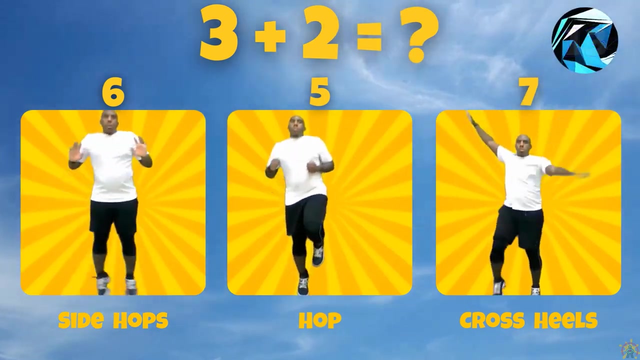 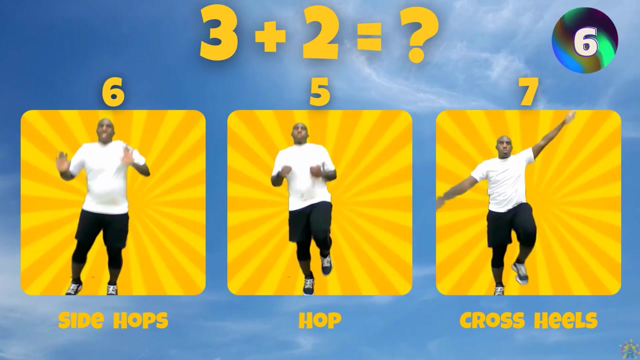 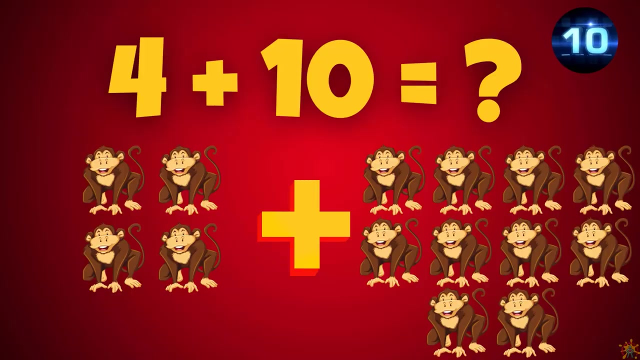 Eight plus four equals twelve. What does three plus two equal? Does three plus two equal six, five or seven? Three plus two equals five. What does four plus ten equal? What does seven equal? What does eight equal? What does nine equal? 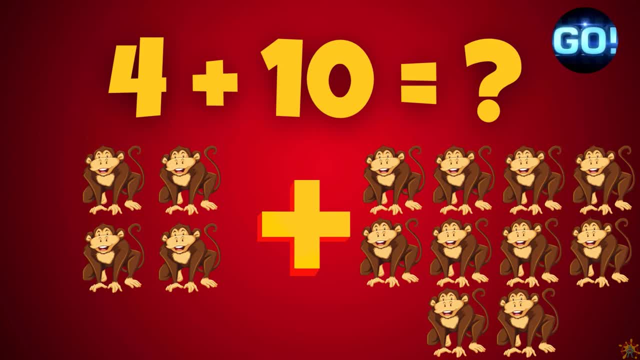 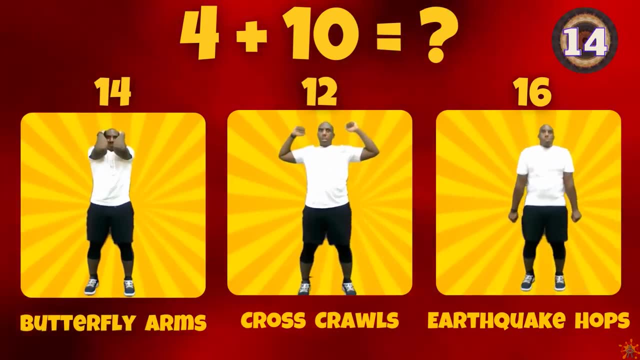 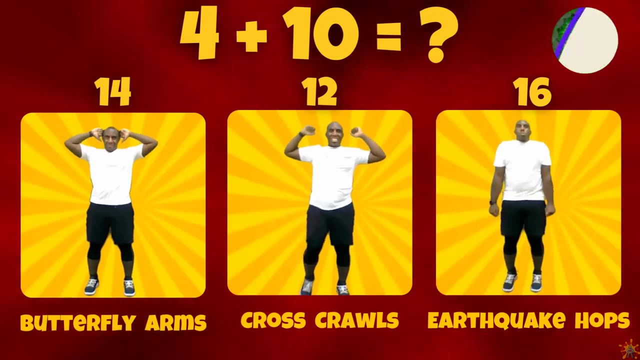 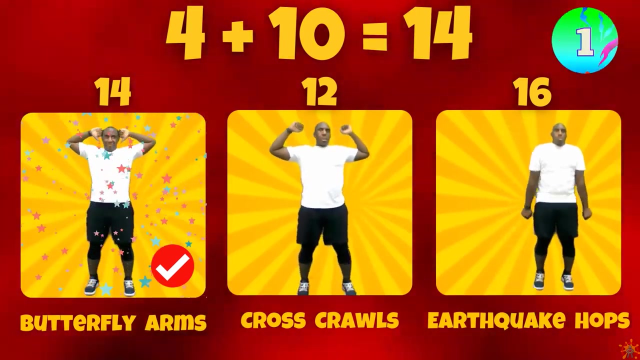 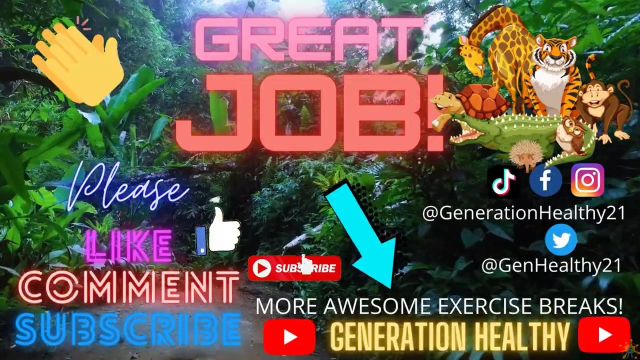 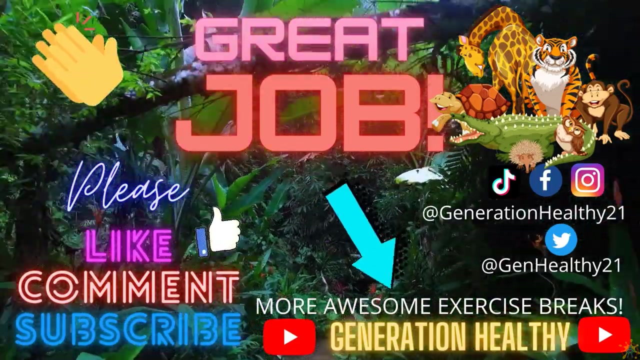 What does ten equal? What does ten equal? Does four plus ten equal fourteen, twelve or sixteen? Four plus ten equals fourteen. Great job everybody. Thank you for playing our Safari Edition game. We will have more cool edition games coming in the future. 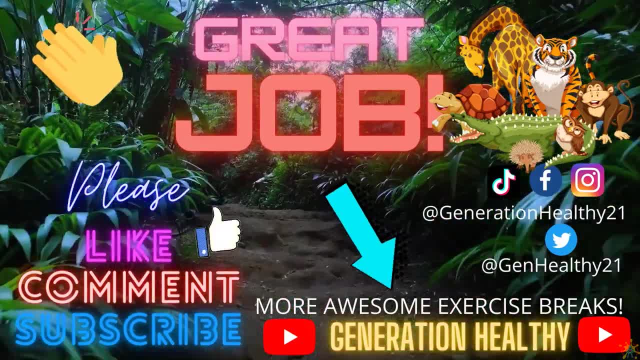 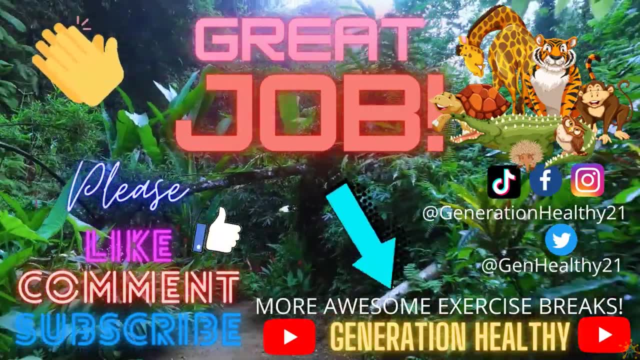 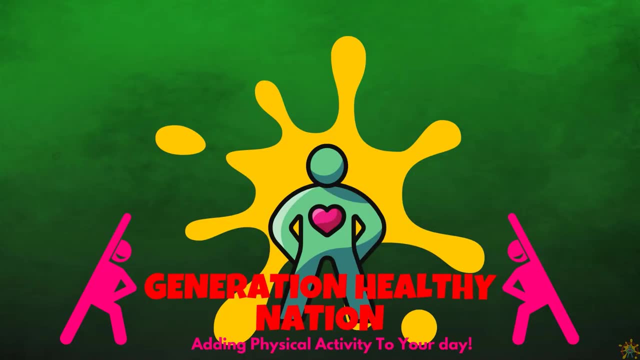 Come back to Moving Time Academy and check it out. If you like other Brain Breaks, check out Generation Healthy on YouTube. We have more awesome Brain Breaks there as well. All right, guys, I will see you in the next video.